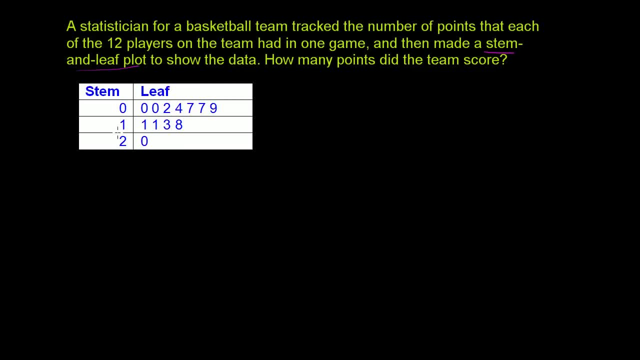 And when you first look at this plot right over here, it seems a little hard to understand. Under stem you have 0,, 1,, 2.. Under leaf you have all of these digits here. How does this relate to the number of points each student or each player actually scored? 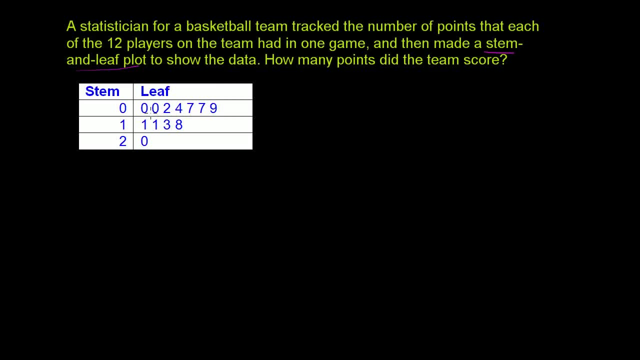 And the way to interpret a stem and leaf plot is: the leafs contain, at least the way that this statistician used it- the leaf contains the smallest digit or the ones digit in the number of points that each player scored, and the stem contains the tens digits. 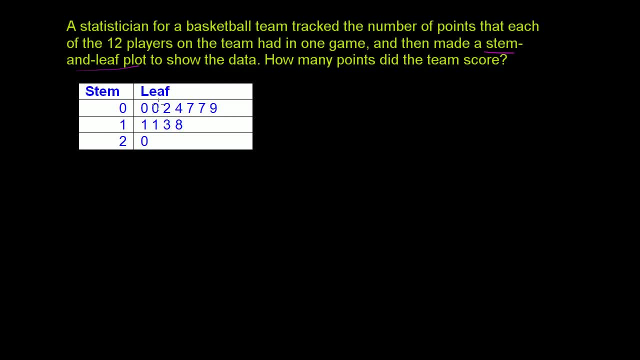 And usually the leaf will contain the right most digit or the ones digits and the stem will contain all of the other digits, And what's useful about this is that it gives a distribution of where the players were. You see that most of the players scored. 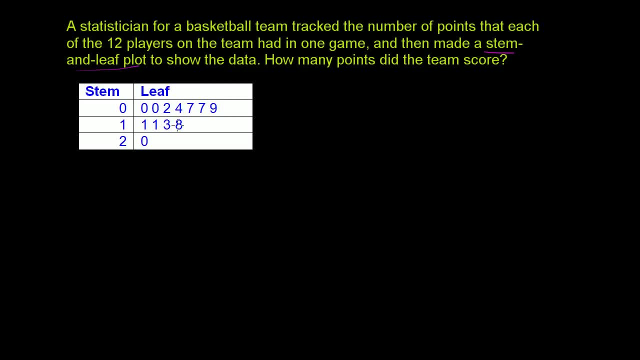 points that started with a zero, then a few more scored points that started with a one, and then only one score scored points that started with a two, and it was actually 20 points. So let me actually write down all of this data in a way that maybe you're a little bit. 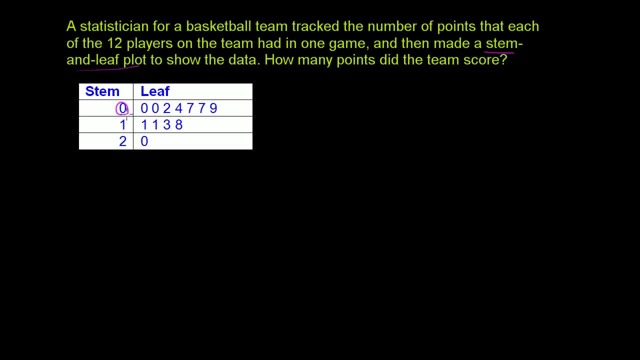 more used to understanding it, So I'm going to write the zeros in purple. So there's, let's see. one, two, three, four, five, six. seven players had zero as the first digit. One, two, three, four, five, six, seven. 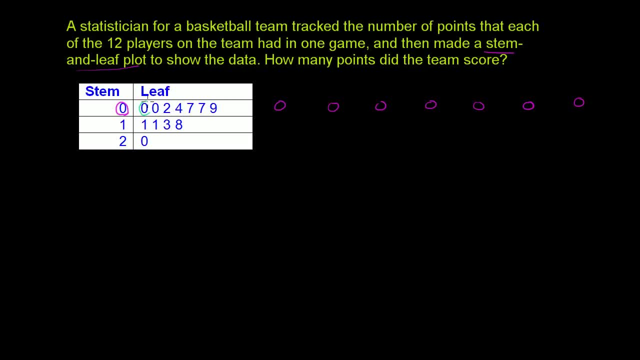 I wrote seven zeros. and then this player also had a zero in his ones digit. This player- I'm going to try to do all the colors- this player also had a zero in his ones digit. This player right here had a two in his ones digit, so he scored a total of two points. 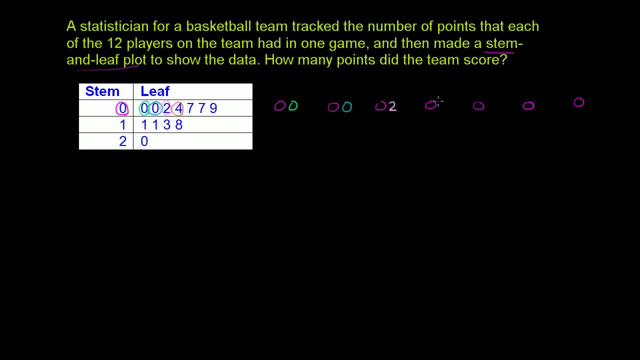 This player. let me do orange. this player had four for his ones digit. This player had seven. Okay, This player had seven for his ones digit. then this player had seven for his ones digit. and then let me see. I'm almost using all the colors. 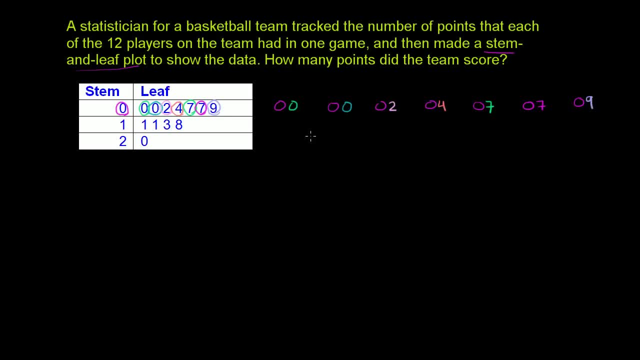 This player had nine for his ones digit. So the way to read this is: you had one player with zero points, zero two, four, seven, nine and nine. But you can see, I mean it's kind of silly saying the zero was the tens digit. 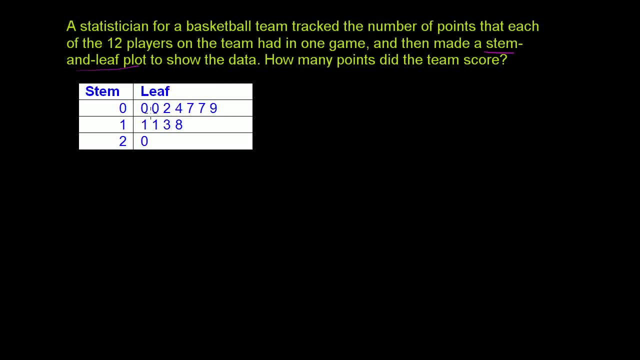 The way to interpret a stem and leaf plot is: the leafs contain, at least the way that this statistician used it: the leaf contains the smallest digit or the ones digit in the number of points that each player scored, and the stem contains the tens digits. 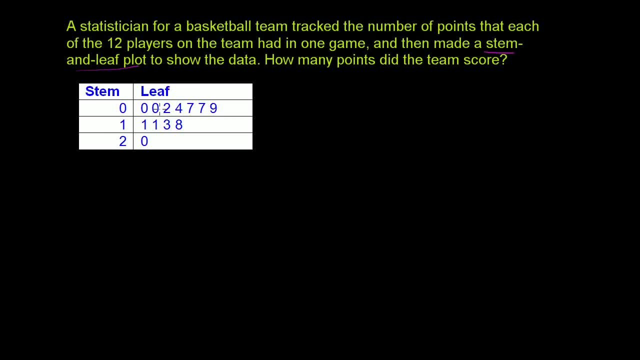 And usually the leaf will contain the rightmost digit or the ones digits, and then the stem will contain all of the other digits. And what's useful about this is it gives kind of a distribution of where the players were. You see that most of the players scored. 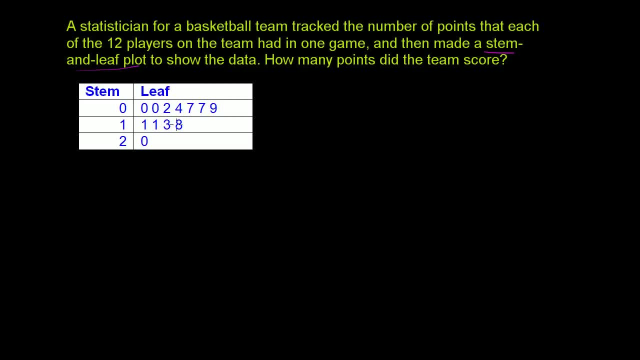 where the players were. You see that most of the players scored points that started with a 0, then a few more scored points that started with a 1, and then only one score scored points that started with a 2.. 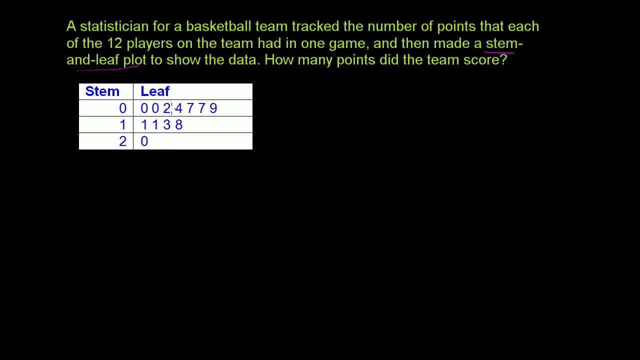 And it was actually 20 points. So let me actually write down all of this data in a way that maybe you're a little bit more used to understanding it. So I'm going to write the 0's in purple. So there's, let's see 1,, 2,, 3,, 4,, 5,, 6,, 7 players. 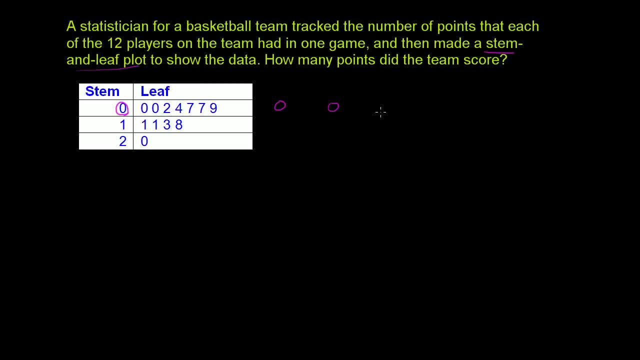 had 0 as the first digit, So 1,, 2,, 3,, 4,, 5,, 6, 7.. I wrote seven 0's, And then this player also had a 0 in his 1's digit. 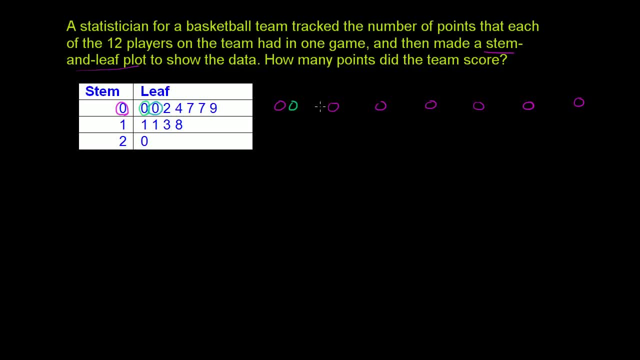 This player. I'm going to try to do all the colors. this player also had a 0 in his 1's digit. This player right here had a 2 in his 1's digit, so he scored a total of two points. 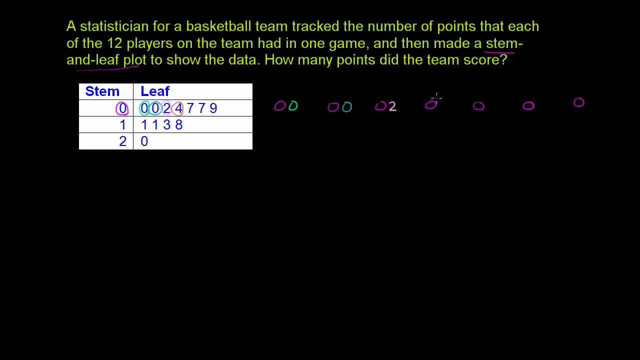 This player. let me do orange. this player had 4 for his 1's digit. This player had a 2.. This player had 7 for his 1's digit. Then this player had 7 for his 1's digit. 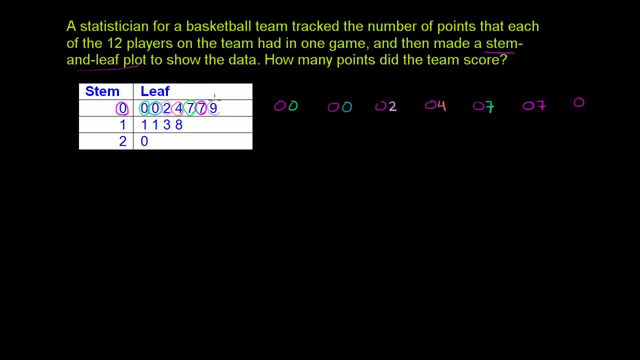 And then let me see- I'm almost using all the colors. This player had 9 for his 1's digit. So the way to read this is: you had one player with 0 points: 0,, 2,, 4,, 7,, 9, and 9.. 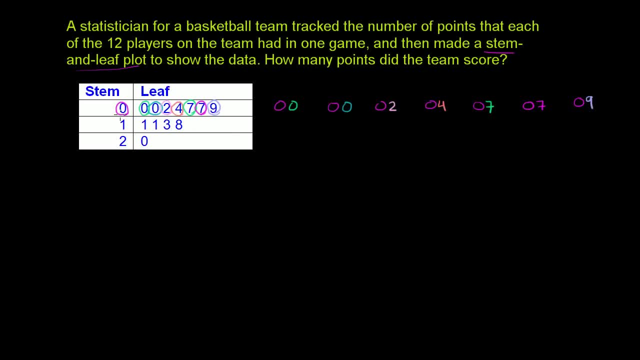 But you can see. I mean it's kind of silly saying the 0 was the 10's digit. You could have even put a blank there, but the 0 lets us know that they didn't score anything in the 10's place. 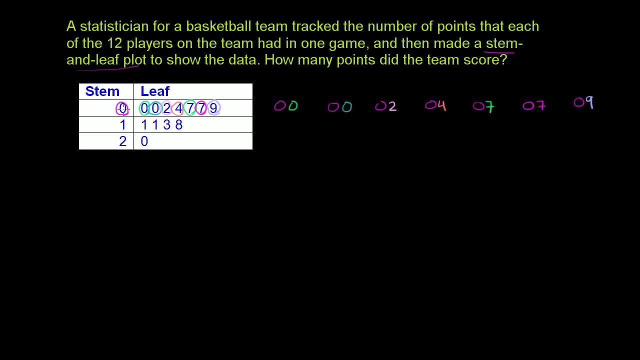 You could have even put a blank there, but the zero lets us know that they didn't score anything in the tens place. But these are the actual scores. These are the actual scores for those seven players. Now let's go to the next row in the stem and leaf plot. 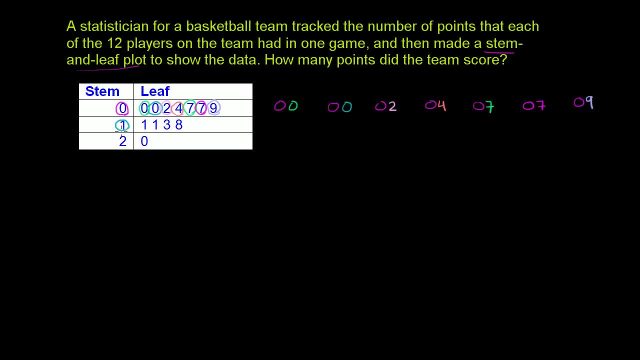 So over here all of the digits start with, or all of the points start with, one for each of the players, and there's four of them. So one, one, one and one. And then we have this player over here. his ones digit or her ones digit is a one. 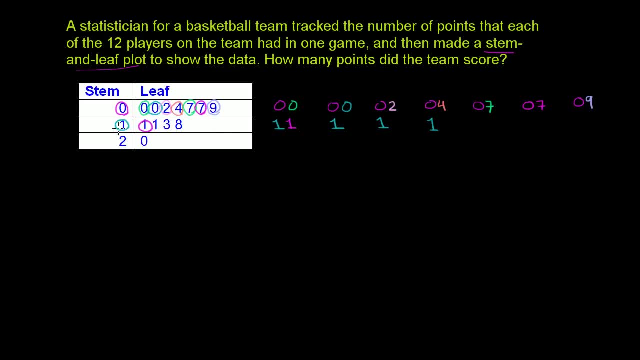 So this player, this represents 11. One in the tens place, One in the ones place. This player over here also got 11. One in the tens place, one in the ones place. This player- let me do orange- This player has three in the ones place. 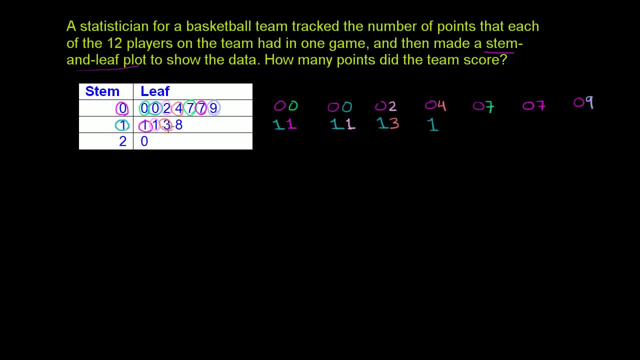 So he or she scored 13 points. One in the tens place, three in the ones place. 13 points, And then I will do this in purple. This player has eight in their ones place, So he or she scored 18 points. 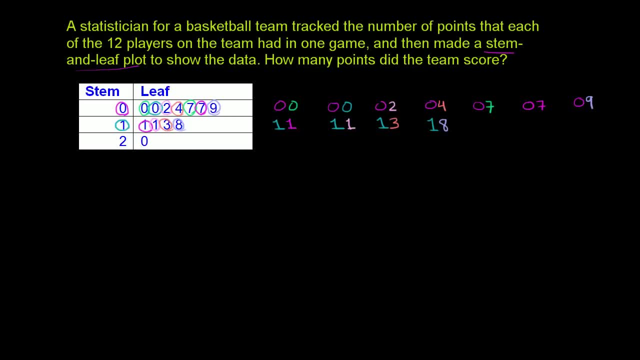 One in the tens place, Eight in the ones place, And then finally you have this player that has two. the tens digit is a two and then the ones digit is a zero. I'll circle that in yellow. It is a zero. So he or she scored 20 points. 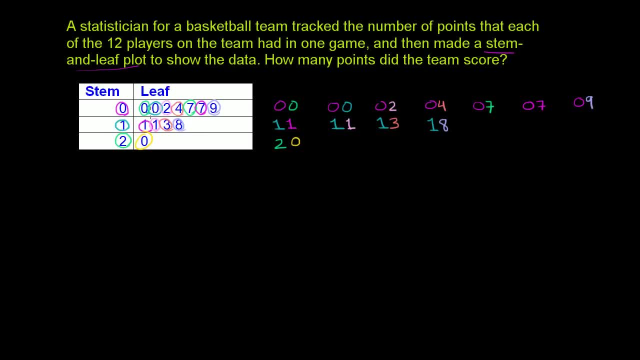 So, using looking at the stem and leaf plot, we were able to extract out all of the number of points that all of the players scored And, once again, what was useful about this is you see how many players scored between zero and nine points, including nine points. 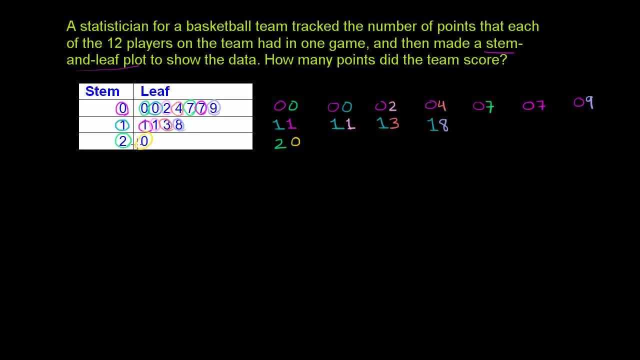 how many scored between 10 and 19 points, and then how many scored 20 points or over. And you see the distribution right over here. But let's actually answer the question that they're asking us to answer: How many points did the team score? So here we just have to add up all of these numbers right over here. 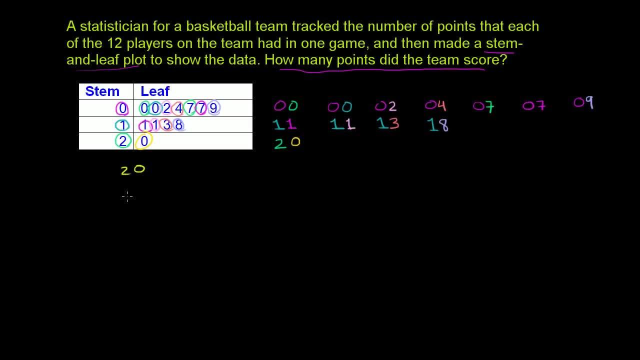 So we're going to add up. I'll start with the largest, So 20 plus 18 plus 13.. Plus 11, plus 11, 13,, 11,, 11, plus 9, plus 7, plus 7 again, plus 4, plus 2.. 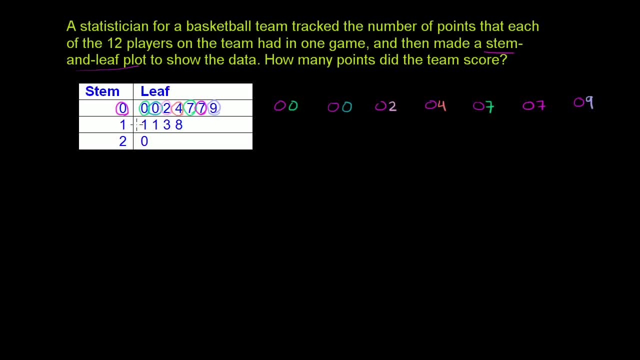 But these are the actual scores for those seven players. Now let's go to the next row in the stem and leaf plot. So over here all of the digits start with, or all of the points start with, 1 for each of the players. 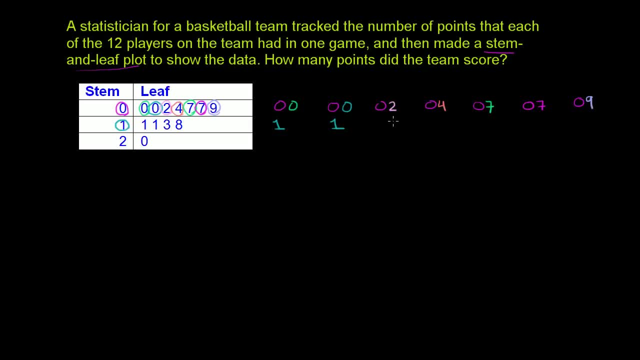 And there's four of them. So 1, 1, 1, and 1.. And then we have this player over here. It's his 1's digit, or her 1's digit is a 1.. So this player, this represents 11.. 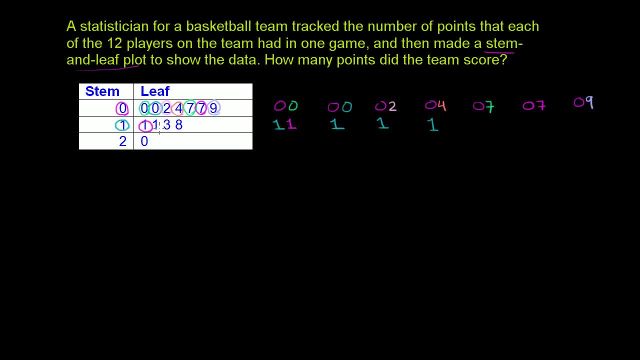 1 in the 10's place, 1 in the 1's place. This player over here also got 11.. 1 in the 10's place, 1 in the 1's place. This player let me do orange. 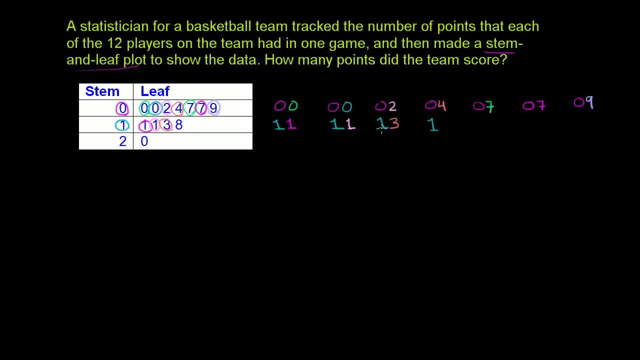 This player has 3 in the 1's place, so he or she scored 13 points: 1 in the 10's place, 3 in the 1's place, 13 points, And then I will do this in purple. 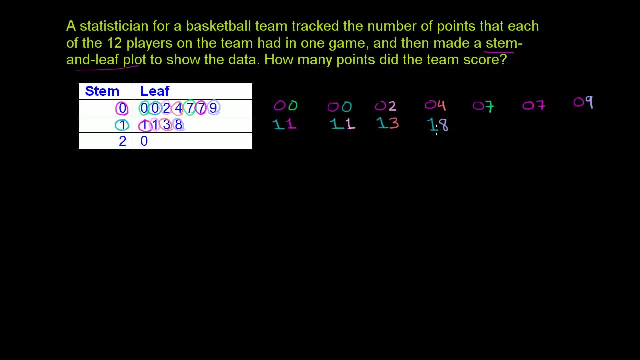 This player has 8 in their 1's place, so he or she scored 18 points, 8 in the ones place, 18 points. And then finally you have this player that has 2, the tens digit is a 2, and then the ones digit is a 0. 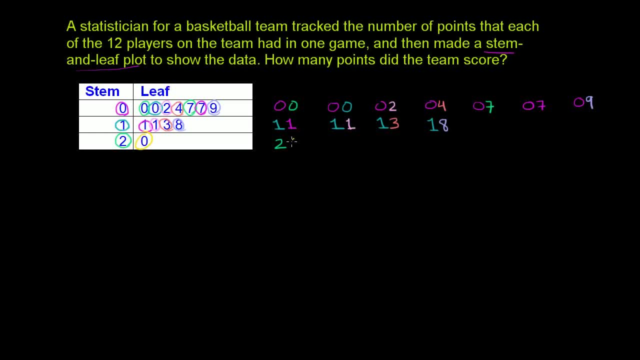 Is a 0,. I'll circle that in yellow. It is a 0. So he or she scored 20 points. So, using looking at the stem and leaf plot, we were able to extract out all of the number of points that all of the players scored. 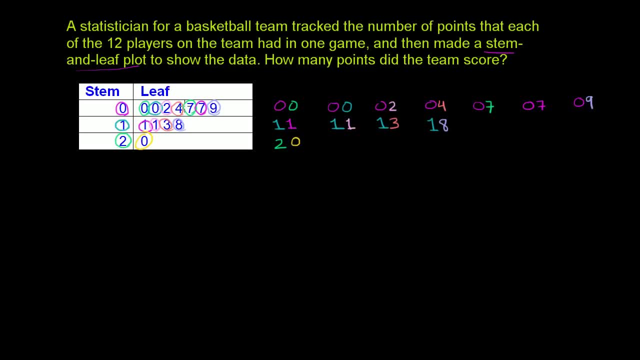 And, once again, what was useful about this is you see how many players scored between 0 and 9 points, including 9 points, How many scored between 10 and 19 points, And then how many scored 20 points or over, And you see the distribution right over here. 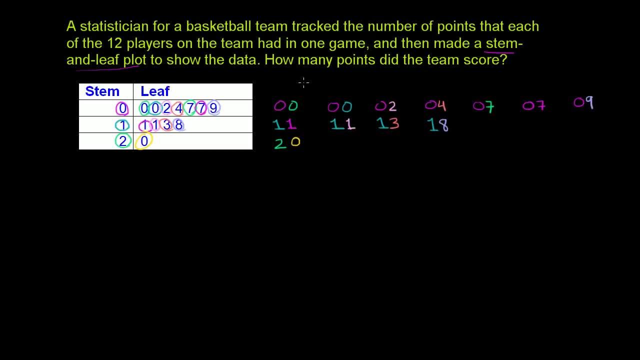 But let's actually answer the question that they're asking us to answer: How many points did the team score? So here we just have to add up all of these numbers right over here. So we're going to add up. I'll start with the largest. 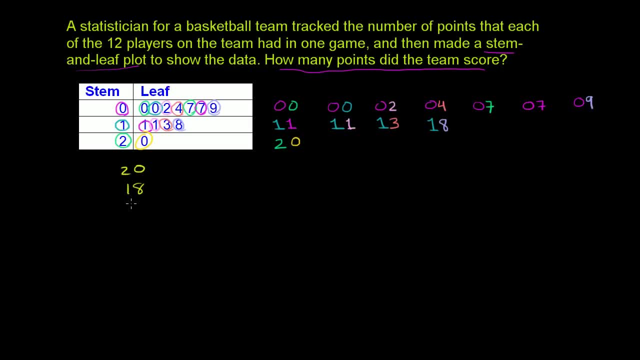 So 20 plus 18 plus 13 plus 11 plus 11.. 13,, 11,, 11. Plus 9 plus 7, plus 7, again plus 4 plus 2.. Did I do that right? We have two 11s, then a 9,, then two 7s, then a 4,, then a 2.. 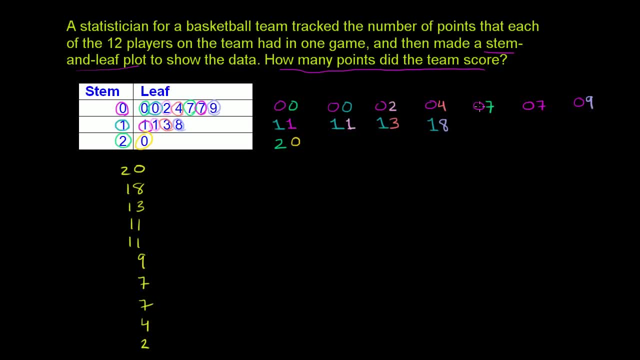 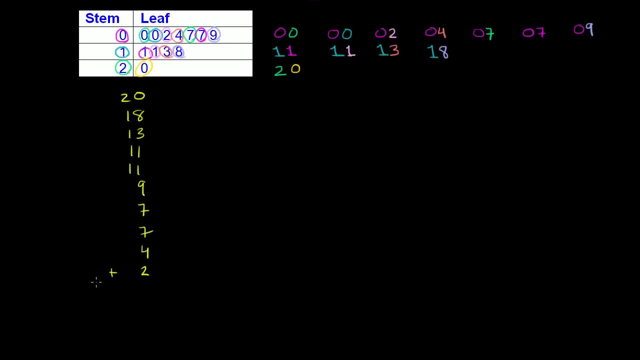 Did I do that right? We have two 11s, then a 9, then two 7s, then a 4,, then a 2, and then these two characters didn't score anything. So let's add up all of these together. Let's add them all up. 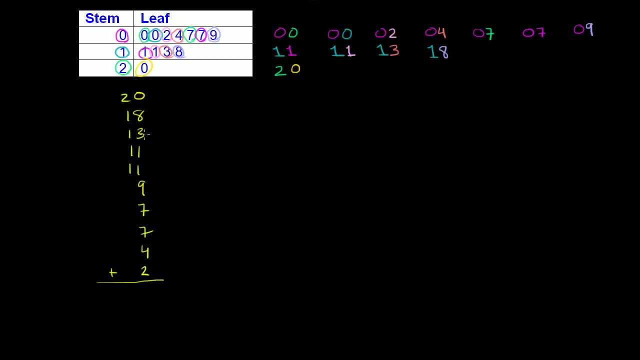 So zero plus 8 is 8,, plus 3 is 11.. Plus 1 is 12,, plus 1 is 13,, plus 9 is 22,, plus 7 is 27,, 34,, 38,, 30, or 40.. 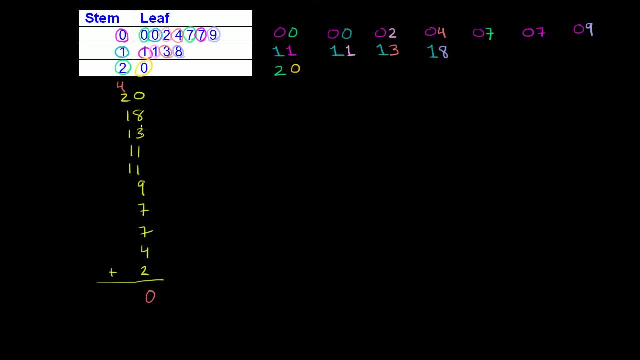 So that gets us to 40.. Let me do that one more time: 8,, 11,, 11,, 12,, 13,, 22,, 29,, 29, and then 29,, 30.. Sorry, 29,, 30.. 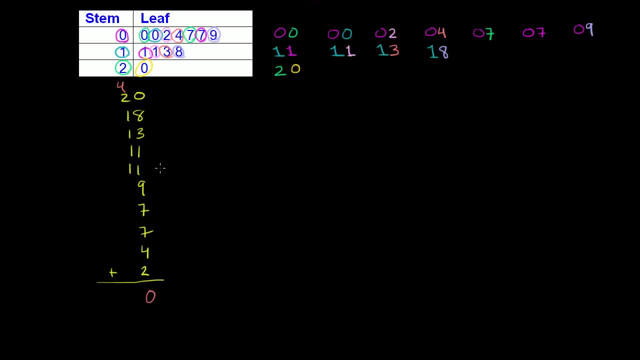 36,, 40, and 42.. Looks like I actually might have messed up. Let me do that one more time. This is the hardest part- adding these up, So let me try that one last time. I'm just going to state where my sum is. 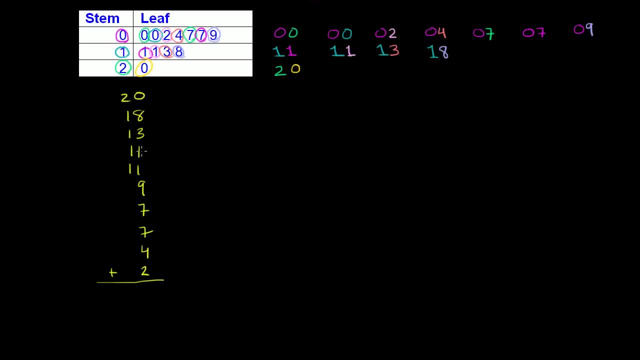 So 0, 8, add 3, 11,, 12,, 13,, 22,, 29,, 36,, 40,, 42. So it's a good thing that I double checked, that I made a mistake the first time. 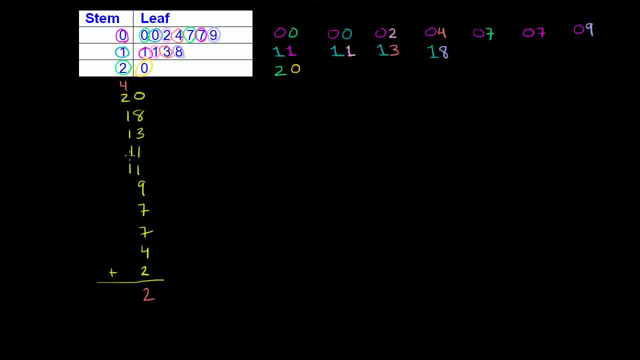 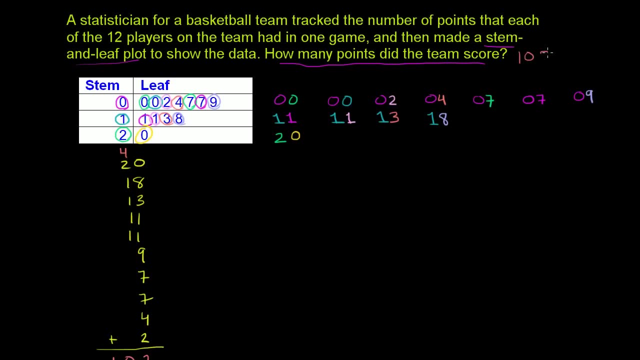 4 plus 2 is 6,, 7,, 8,, 9,, 10.. So we get to 102 points. The team in total scored 102 points.